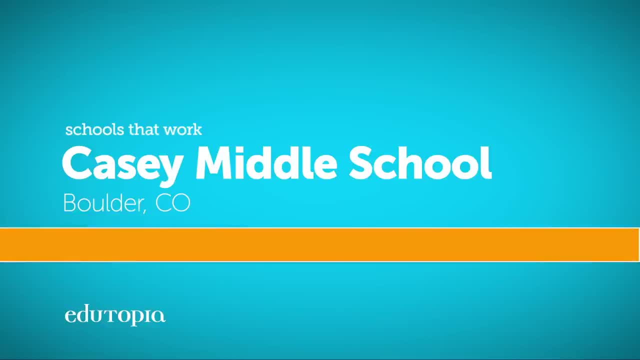 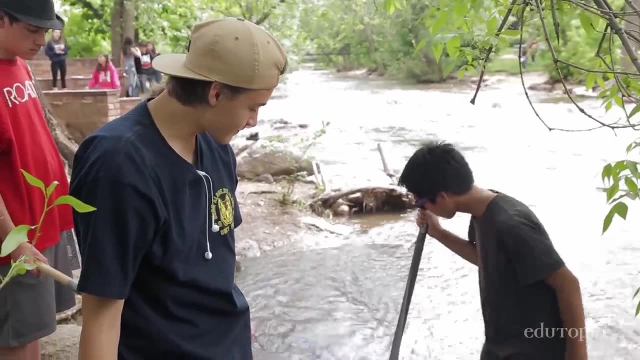 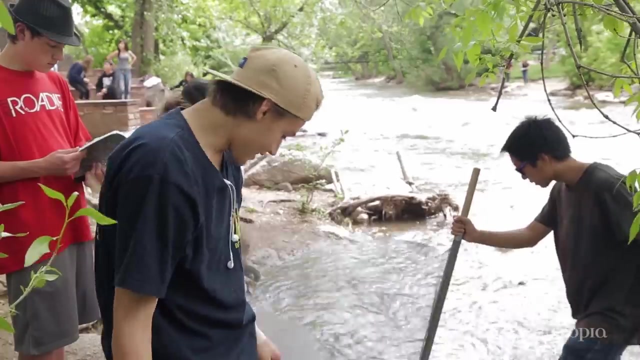 This is still settling, but we found a lot of little organisms, So cool. The real question we're trying to answer here is if it's safe to tube in the water, because I swim here every summer and I just realized how dirty it was. When we design a science lesson to be an inquiry-based, 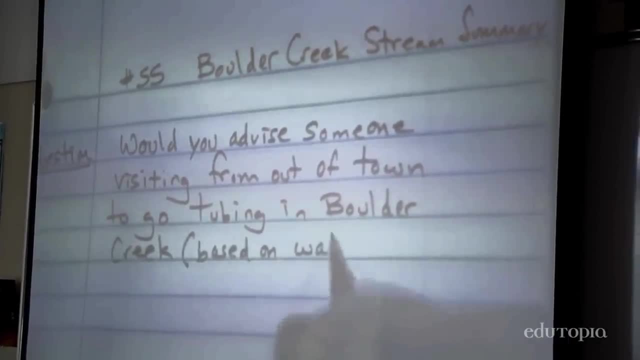 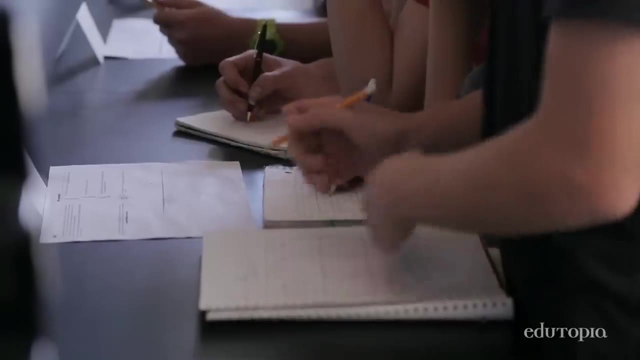 lesson. we start everything around a central question That may last for one class period or a series of class periods, And then they work through some experiment and conversation, perhaps some reading, and they work together And the answers are always just a little bit. 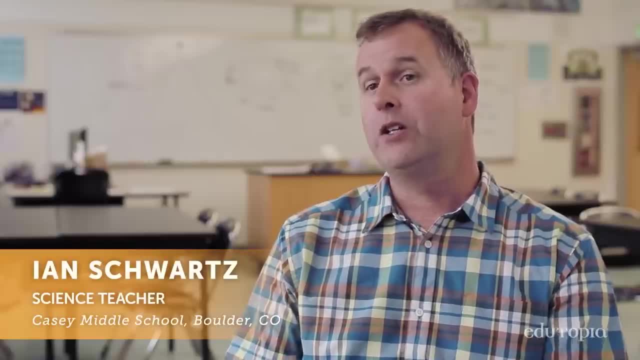 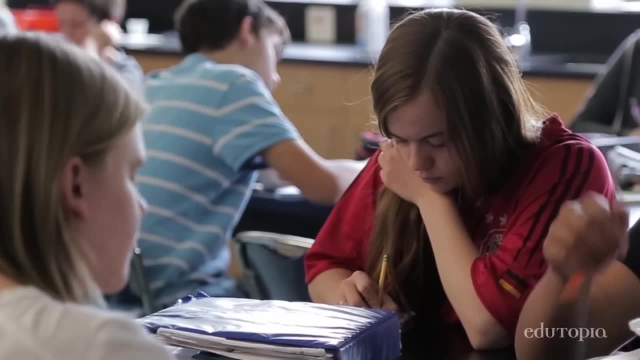 out of reach for the kids until they really reach a point where they have this sense of discovery. Each of you are going to be in a group where you're going to sample one parameter down at the creek And then you're going to make a infographic about your parameters. So for 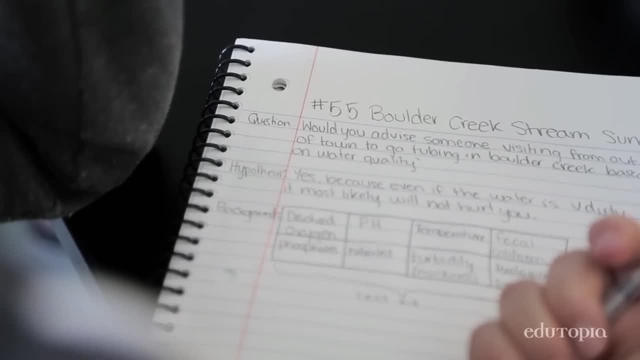 example, maybe it will be temperature and turbidity, And then, ultimately, what you're going to do is you're going to go to the water and you're going to go to the water and you're going to have to decide, And your final prompt is going to be answering this question, Would you? 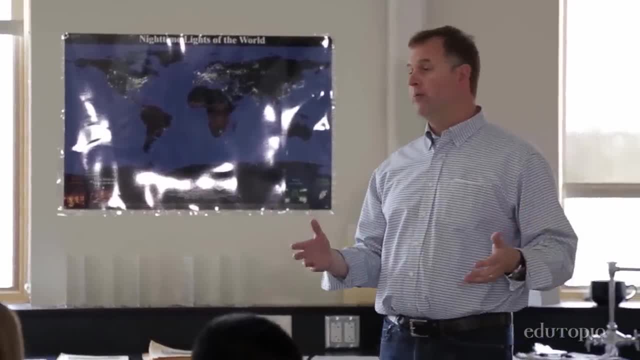 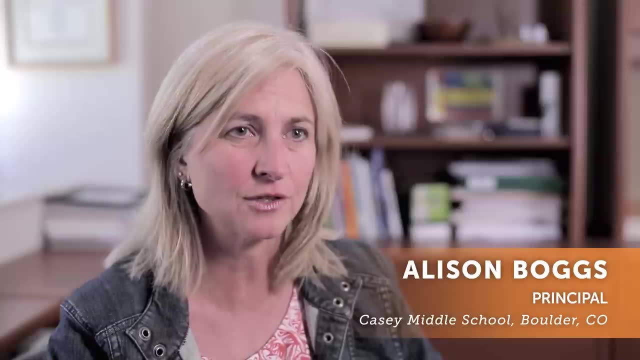 recommend to your friends coming from out of town that they go tubing in Boulder Creek. If you just ask a question and then gave the answer, it would be the same as if you just read the textbook. So we don't like to do that. We like to ask the question and then give a lot of 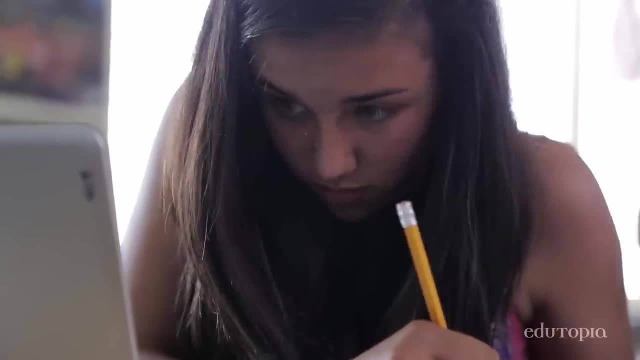 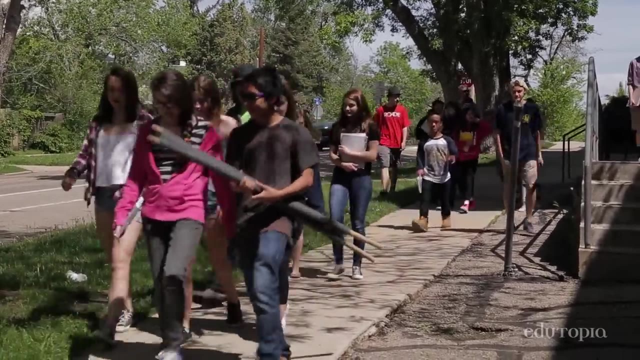 different experiences, both through media, through discussion, through research, so kids can start to answer that question themselves When we actually go down to the creek. it's an exciting experience. It's an exciting experience, It's an exciting day for the kids. We've talked up the idea that we're really in an outdoor 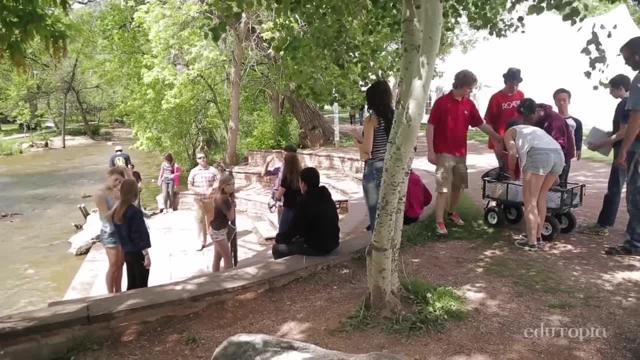 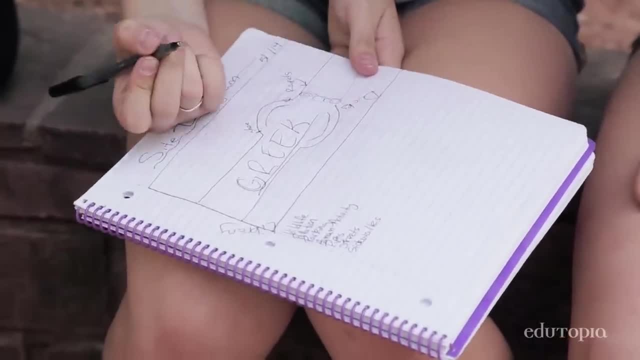 classroom. Let's find a spot and let's sit down and start working on our physical survey of the area- everybody. so you'll work on your map first- And suddenly they're looking at it through a different lens. They're looking at it through a lens as a place where we're now going to be. 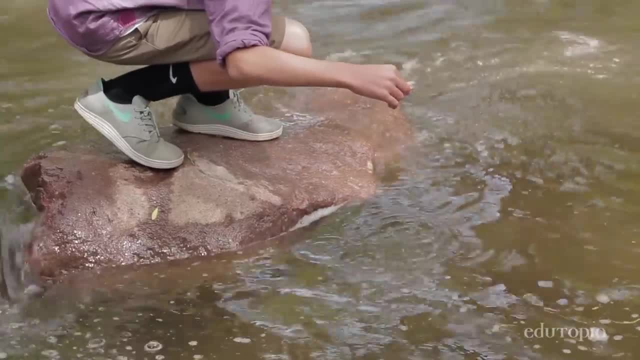 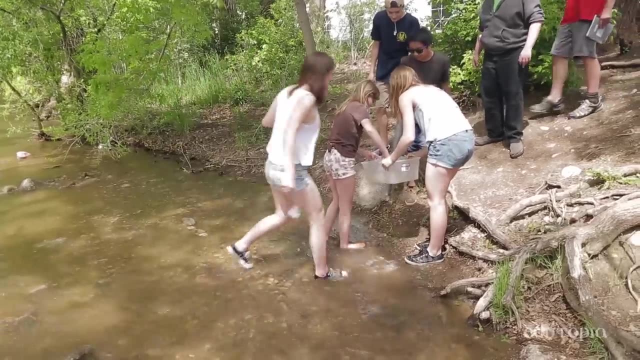 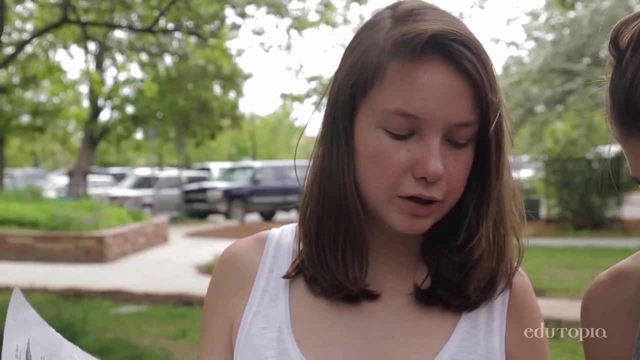 doing some sampling and some scientific thinking. If the water appears clear, Is it clean? And then, if it's not clean, what does that mean? Mr Schwartz gave us bugs that can live in healthy water and bugs that can live in unhealthy water.